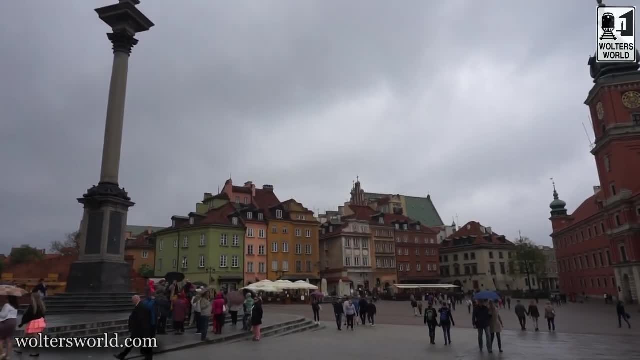 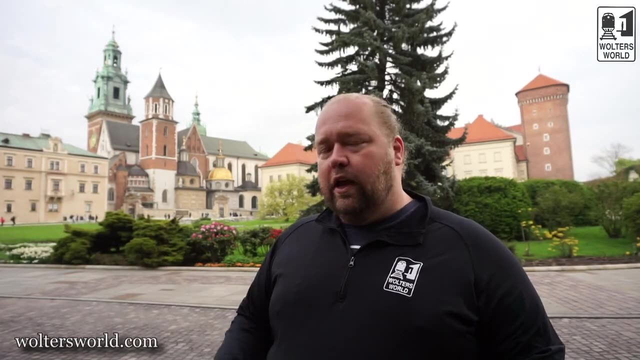 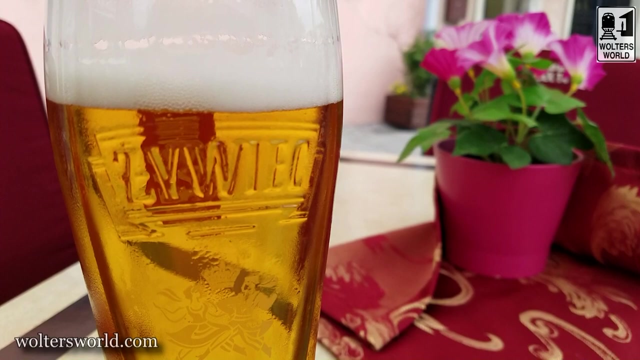 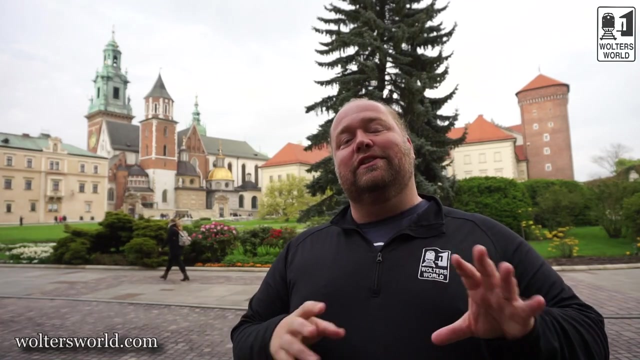 The first time I came here was like 20 years ago. You know, I was a young guy and with my buddy we're doing our backpacking through Europe thing and I was here and I heard like dwa was two, and then there's piwo, but they were saying something else: piwa. I'm like I go and I go, dwa piwa. haha, dwa piwa, which is two piwo because two beers, because it changed it. The guy was so happy. He's like: oh, my God, Fornan, you said it right with a double And he gave me two free beers instead of just two beers. It's pretty funny. So if you can learn just a few words before you come, it will make things a lot easier and the people do open up a lot because they can be super friendly. 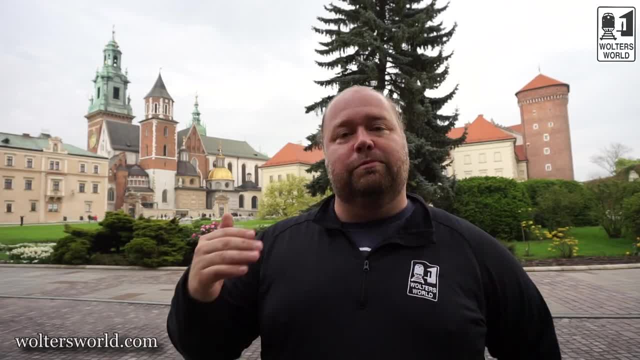 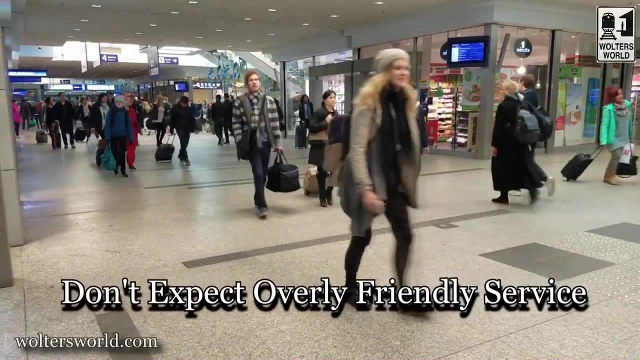 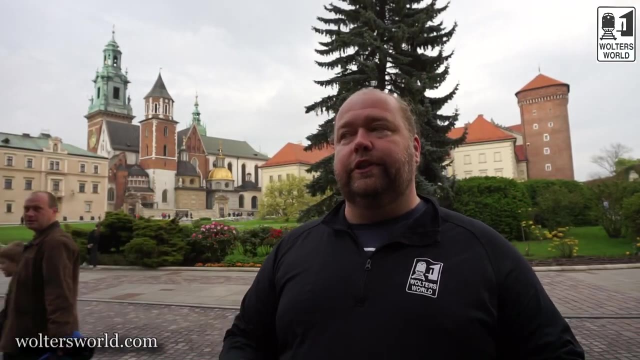 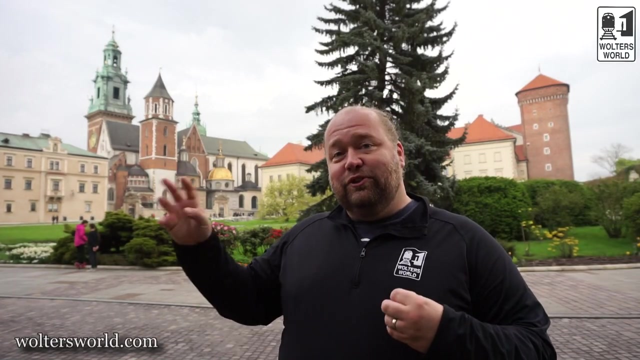 Here. but I think in general for service in Poland, don't expect super lots of service. You'll see a lot of dour faces and things like that. The service is kind of that kind of thing, but it is one thing to kind of got to look out for Now. next thing I want to talk about is money. Coming to Poland is cheap. I'm not saying affordable, I'm saying it is a cheap vacation. And think about it. You can hit beaches in the north and go skiing in Zakopane and the Tatras Mountains in the south. in winter You can see the Missouri Lakes. Like I said, go to Warsaw. here in Krakow eat, drink, make merry at a super great price. 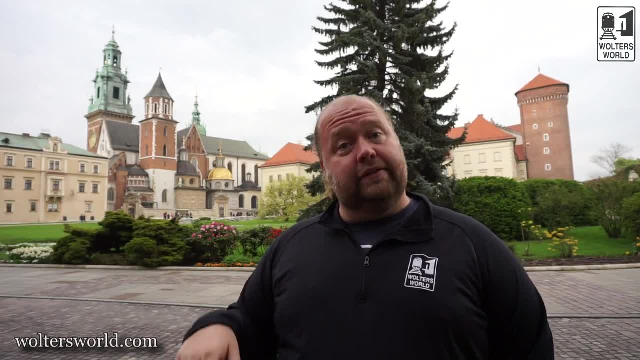 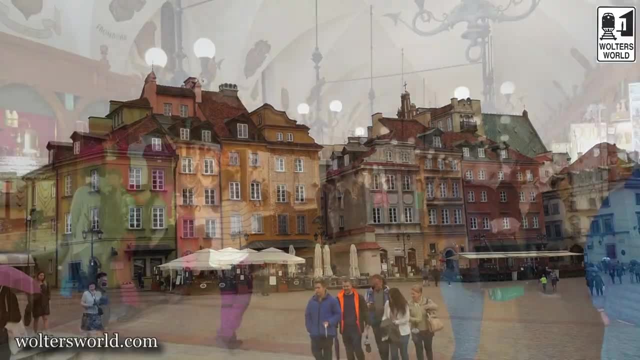 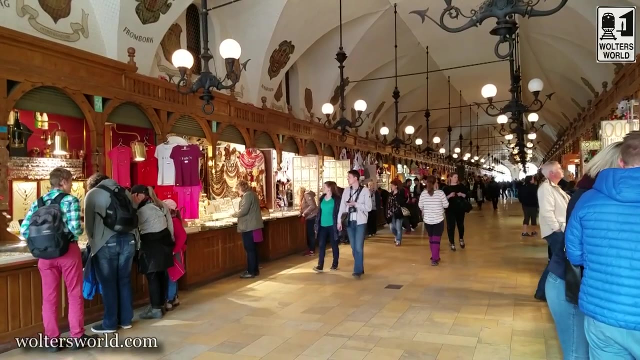 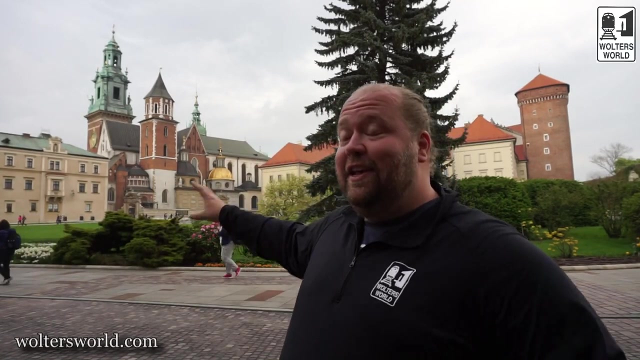 So I would say, like in terms of going out to eat, I would say it's, you know, 30% less than in the US, 30% less than like Germany and stuff like that. So I've been very happy with the pricing that's here, though the service sometimes a bit off. Another thing you might want to know is in terms of during the- during the working hours, normal working hours- your stores still until eight, maybe nine o'clock The weekends. they might close. early Sundays they might all be closed, So your Sundays are going to be seeing beautiful churches and stuff like that. Here in Poland there's a lot of really cool places to visit Now in terms of money, when you are here. this 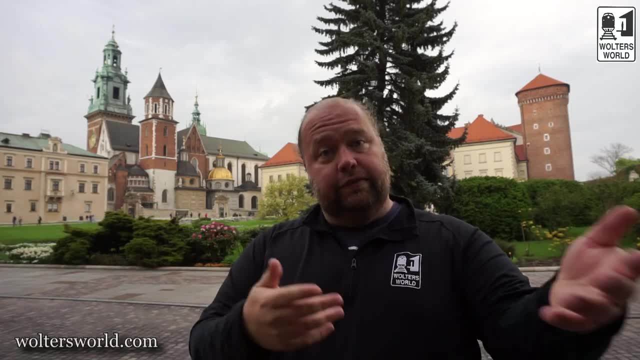 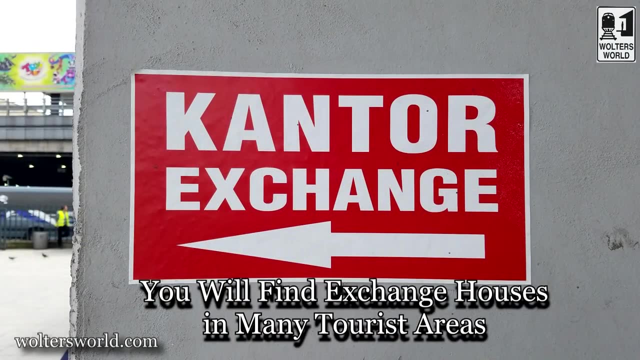 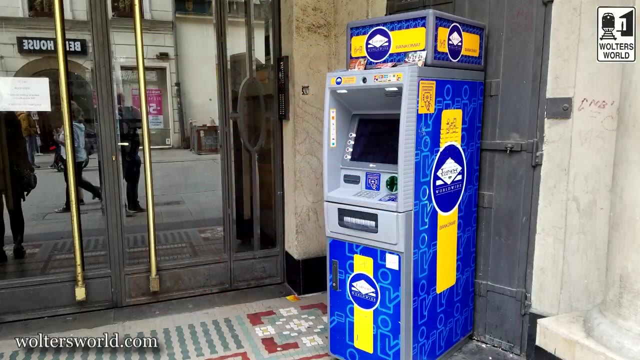 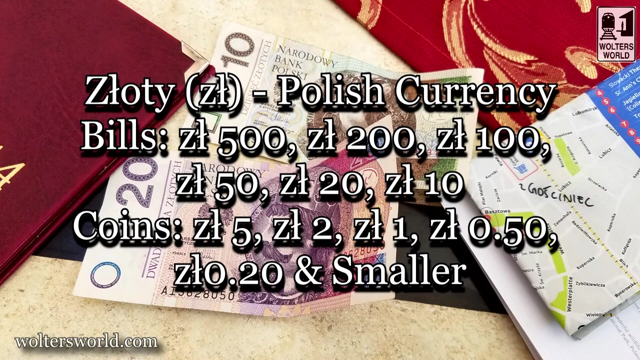 is: yes, they're part of the European Union And so you'd get like a Schengen visa. if you need a Schengen visa, you'd be using that when you come here. But in terms of money they use, they don't use the euro. Okay, they have the swati. you'll see, like a ZL- It's about four to one- to the dollar or the euro. to give you a rough idea what it is. And you know, if you're looking at the price, you can get the money anywhere. There's lots and lots of ATMs And there's multiple bills. there's, you know, the 10,, 20,, 50,, 100, and so on. You have those bills and they're smaller coins, like a five, five swati coin. 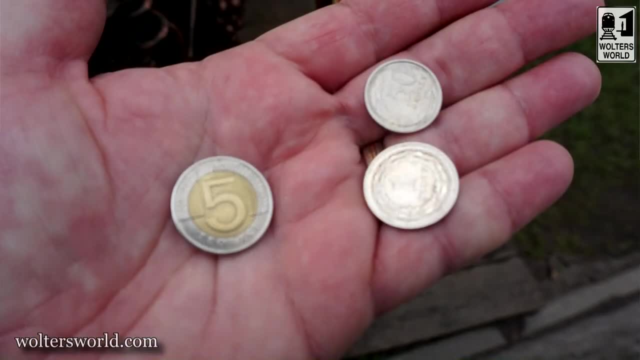 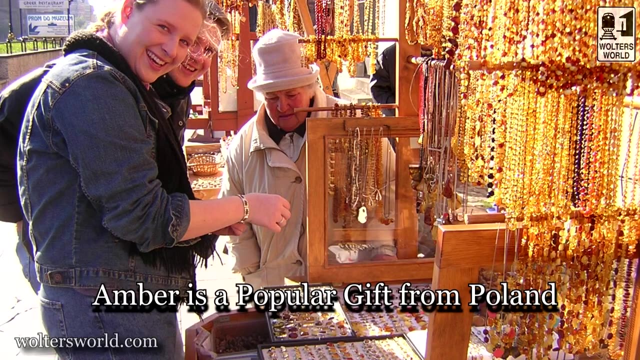 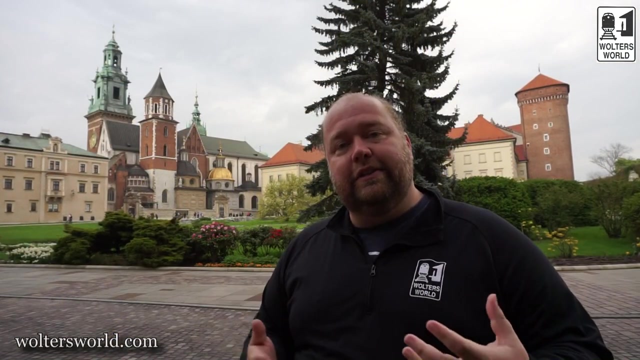 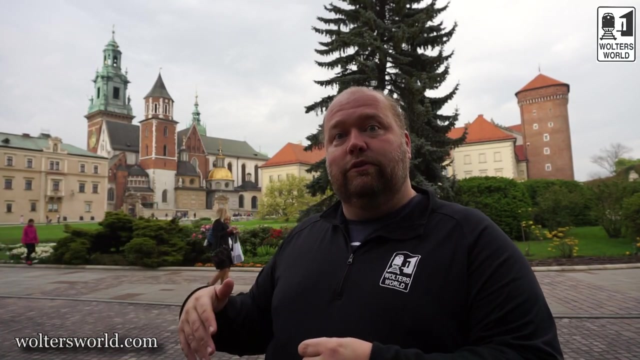 Two, one swati coin, things like that. But the thing is, if you're going to pay for stuff with cash, if you're going to need more than like 20 swatis and change, they're going to ask for a smaller bill. So try to get the smallest bills you can. I know when you go to the ATM they give you like hundreds and 50s, But it's hard to find stuff that costs that much, except you're going out to eat or something like that. So try to break it into smaller bills. And if you do get smaller bills and say you pay with 100, and they give you change, save those smaller bills for when you're going to get a kielbasa, you know the sausage, or going to get you know a beer someplace. 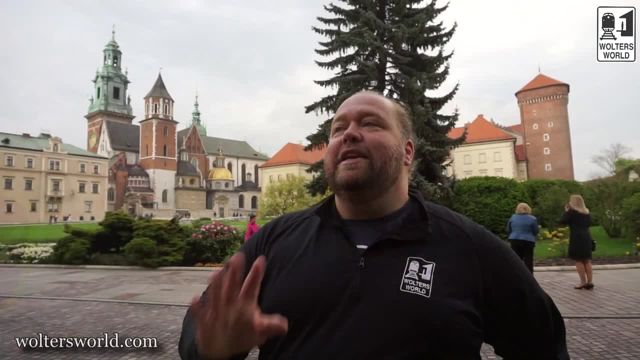 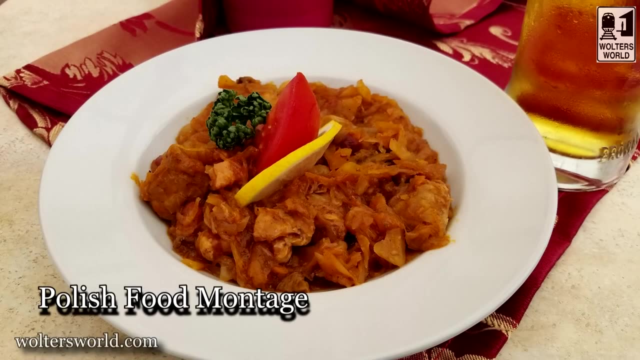 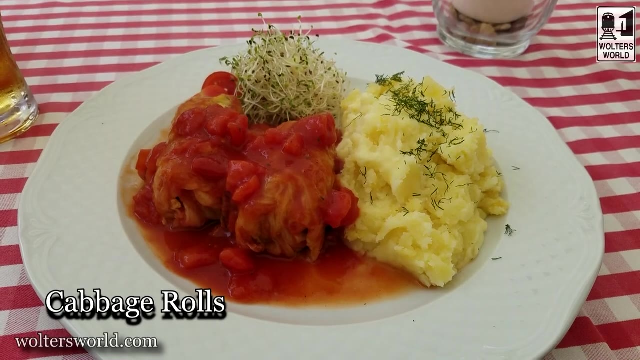 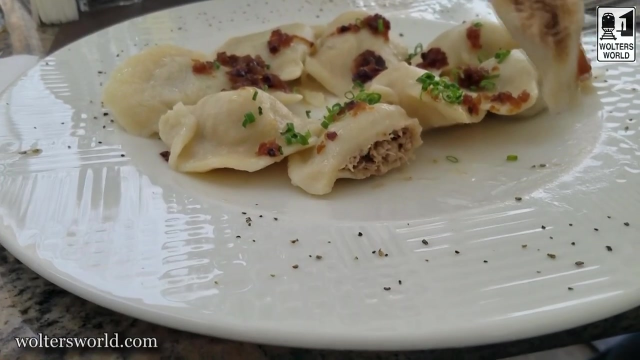 Things like that. So you have the smaller bills out there. Okay, Now other things you might want to know when you come here, when you're going to be eating here. I have a whole video on what to eat in Poland, But some of the bigger things you need to know- meat and potatoes is your big thing here. Pork, potatoes, potato pancakes, a lot of cabbage. of course you're gonna have the pierogi, which is like their version of a kind of ravioli. It might have cabbage and mushroom in it, or it might have some cheese, or might have meat with onion in it. They're actually really good. If you come in the summer, a lot of times you can get them with fruit inside, And they love their sour cream and cottage cheese stuff, And you'll see weird cheese. 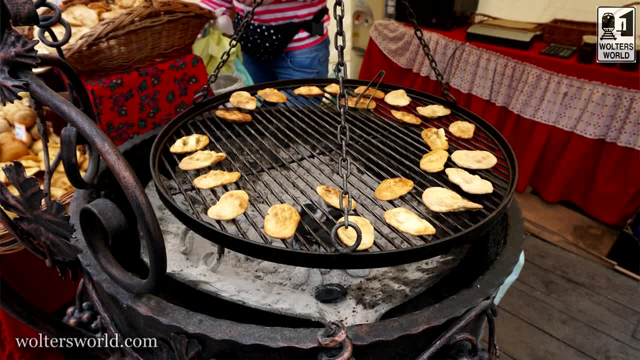 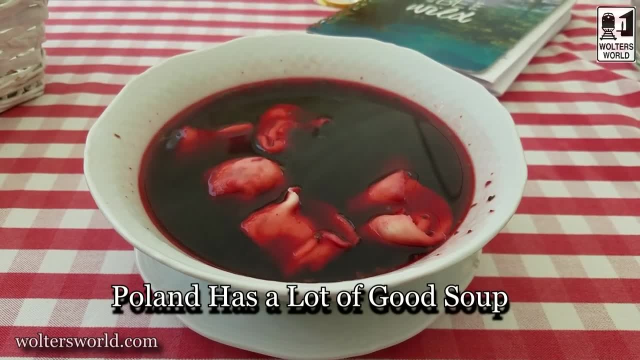 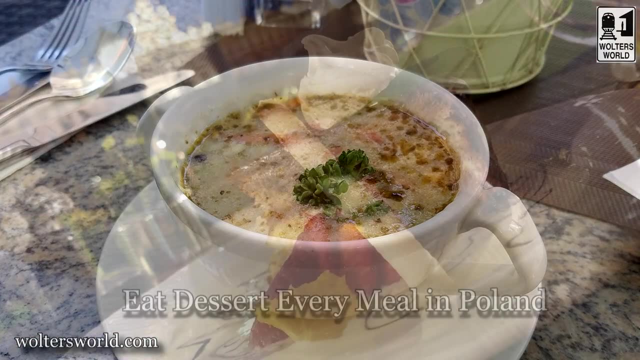 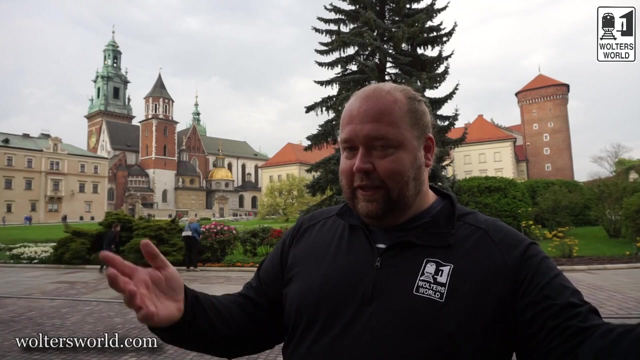 here that look, you know funny, you'll have them grilled for you and eat it with jam. It is really good. But it's a lot of meat potatoes kind of stuff when you are here, So it can be kind of heavy. You do have a lot of like international kiosks that are here, But in general, just think meat potatoes- you know grandma's kind of food. you'll be okay. Also, when you're here to when you're drinking here, you can drink the tap water, though it might not taste very good, but you can drink the tap water. It is the European Union, Okay. so you do drink the water, But you don't see people drink it very much. What you see people drinking a lot actually is tea. 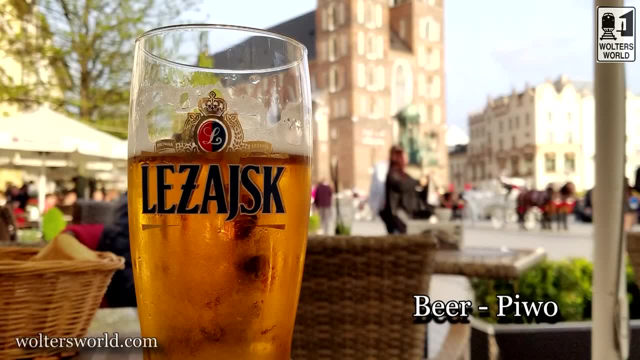 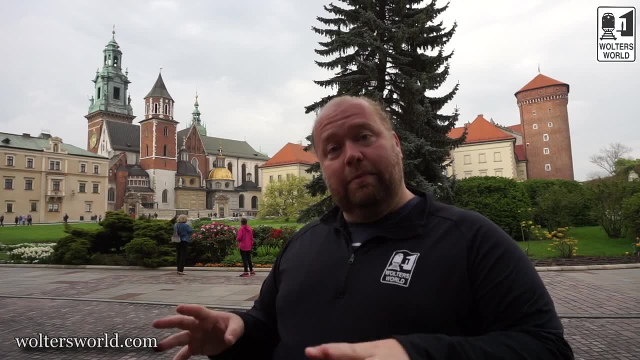 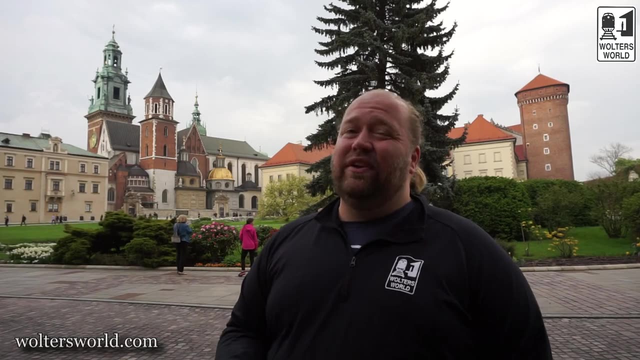 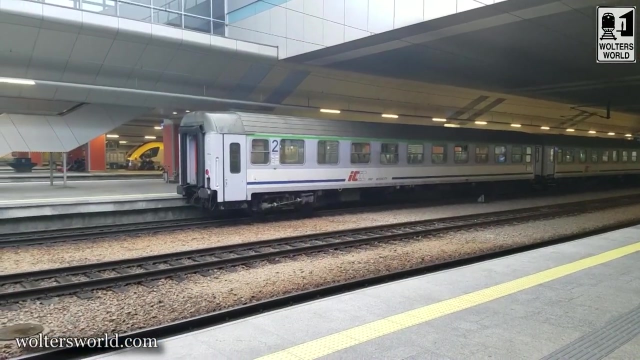 Okay, they like it, They like their tea here. They also like their beer and, yes, the vodka. But all those three things are fine. That's kind of your more traditional drinks when you are going to be here. Other things you might want to know about when you are here. in terms of transportation, train system goes lots of places. There's not a lot of those super fast trains you know like in Germany and France. You don't have that too much. You have a lot slower trains when you're here. A lot of people. there's a big bus network and the buses are super cheap when you are here to get you around places. If you're traveling on the weekend with trains, they have weekend tickets you can get to save a little bit more money. So you're. 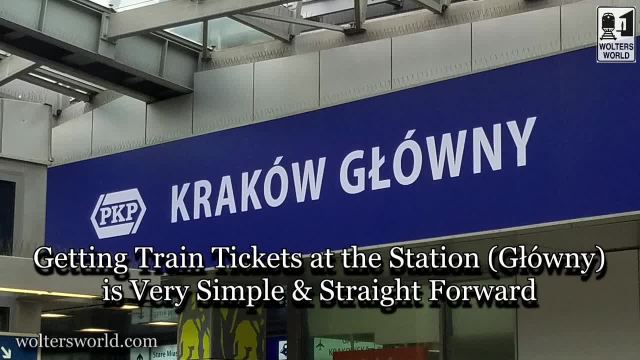 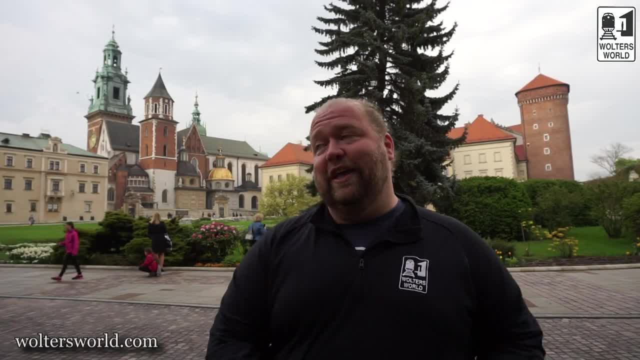 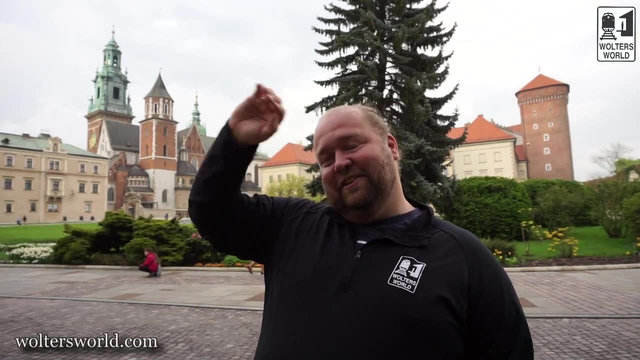 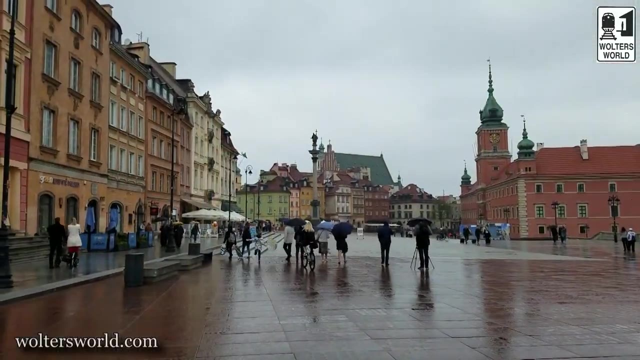 going to do like a round trip to places. you're going to be okay In terms of places to visit when you are here, but there are places while we're visiting, Like I said, skiing in the Tatras and go to Zakopane in the winter for that, Going to the Missourian Lakes and seeing those things. there There's, you know, the castles that are around the country randomly, which is kind of funny. The beaches in the north, obviously only in the summer, And I would say June, July, August, more July and August are the best months for that. outside It might be a little cold, unless you like that polar bear swim kind of stuff. Warsaw, which was destroyed during the war- they've 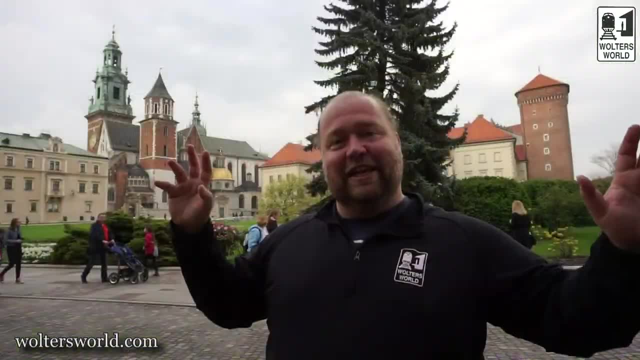 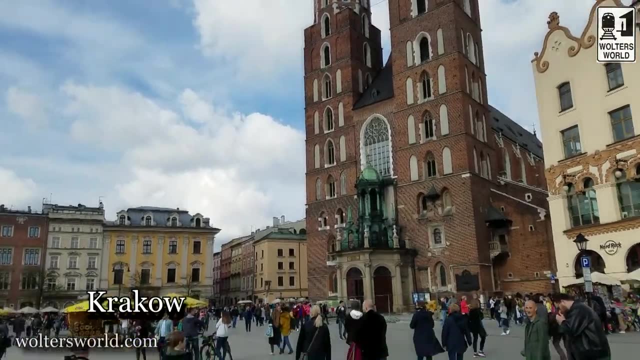 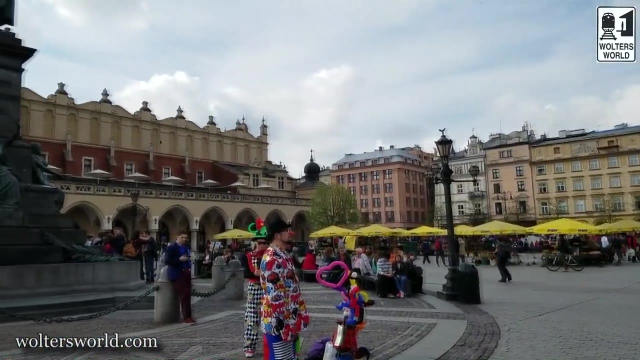 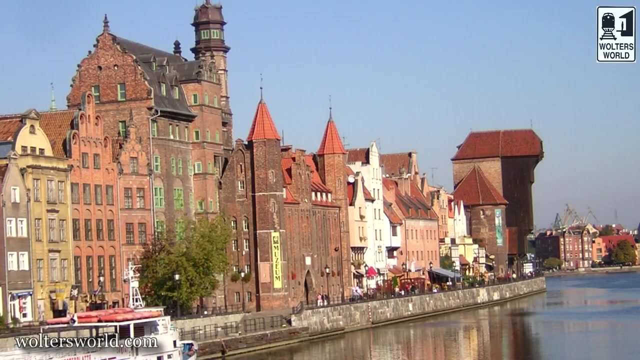 rebuilt the center so it looks just like it used to, But outside that it's all steel and glass. You have that here in Krakow. You have the- you know the Royal Hill. you have Wawel Hill here. You can see the cathedral and all the stuff here. There's actually a Da Vinci here in Krakow. you can check out. The town square here is beautiful. But if I'm talking about beautiful town squares, you've got Wroclaw, which got a beautiful town square. Maybe you go see the old town of Lublin. There's a lot of different places around here. Actually, one of my other favorite places is Krakow. My other one is Gdansk, in the very north. You go there, the Neptune statue and see those things. There's a lot of cool things to see when you are. 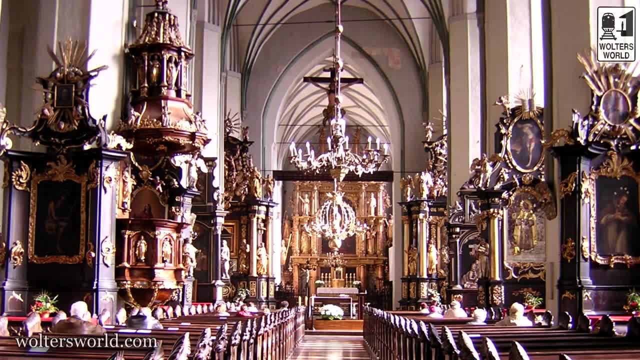 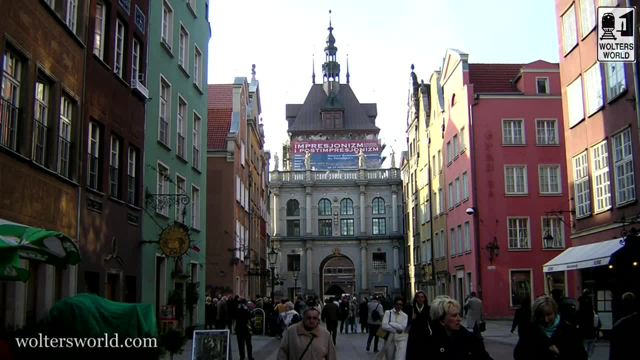 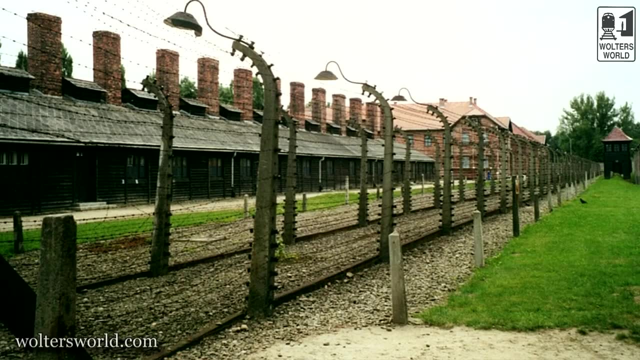 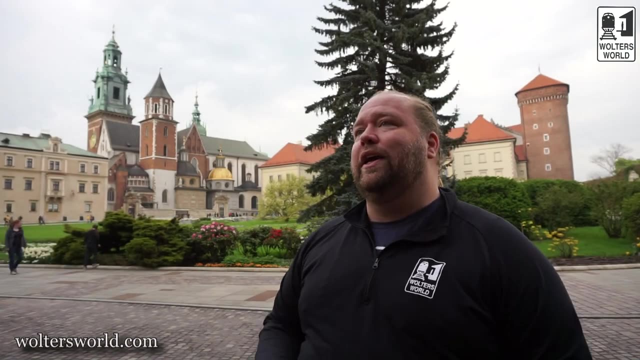 here, But you will be going around because they're kind of spread out of the country. So it will take you some time doing that. And the thing is, if you're looking at tourism, there's not a lot of tourists that come to Poland. Now there's a lot that come to Krakow. There's about 10 million a year that come to Krakow For good reason. This city is gorgeous And, yes, you can get. you can go see Auschwitz and Birkenau- the worst concentration camps out there. You can see that. But you also can go see a salt mine where they build a city inside the salt mine. It is kind of cool that way, And so you have all this really different kind of stuff when you come here. And, yes, you will see the communist architecture. 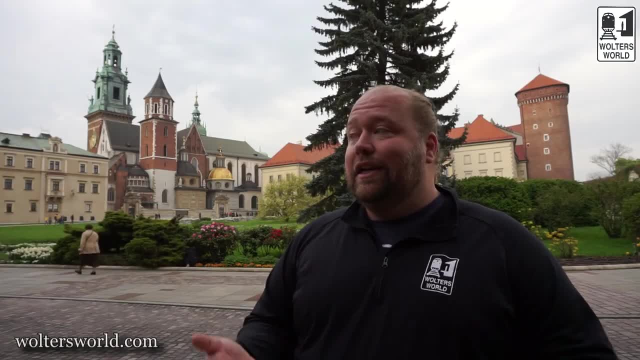 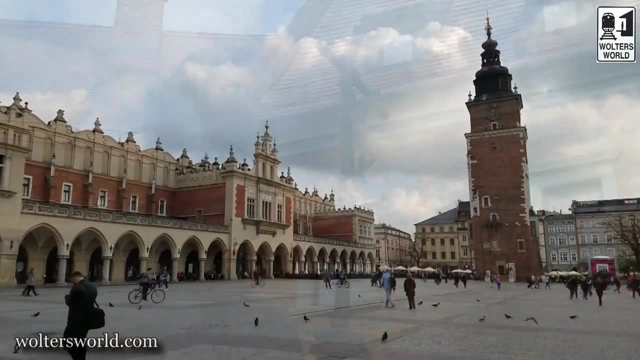 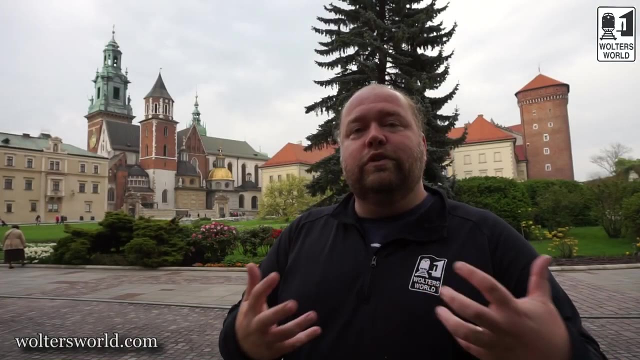 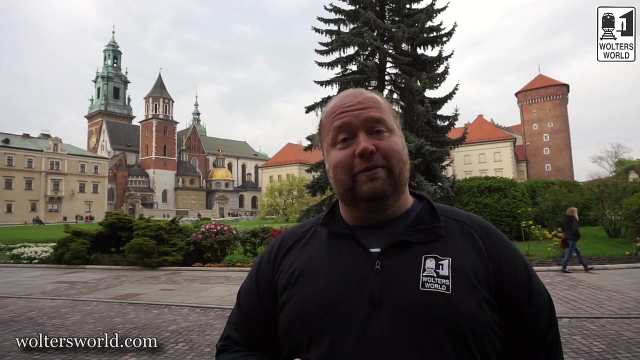 the square built. you know the rectangles that everyone lived in and stuff like that, Because a lot of the country really was destroyed during the war. But the people are very proud of their country. They've really worked hard to rebuild a lot of destroyed areas. So when you see the historic parts of town now Krakow has been lucky. It wasn't really that it wasn't really destroyed very much. But other places, when you see it rebuilt up and you learn about the Warsaw uprising and things like that, you really get proud for the people here, how much they've overcome, And you'll see that in the people. They are very proud of themselves when they are here. Some other things you might want to look at in terms of when you come here: toilets.